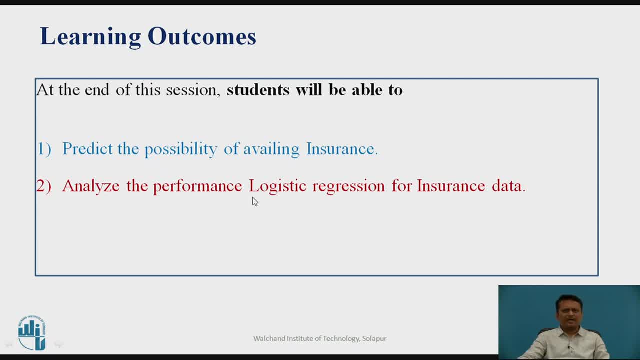 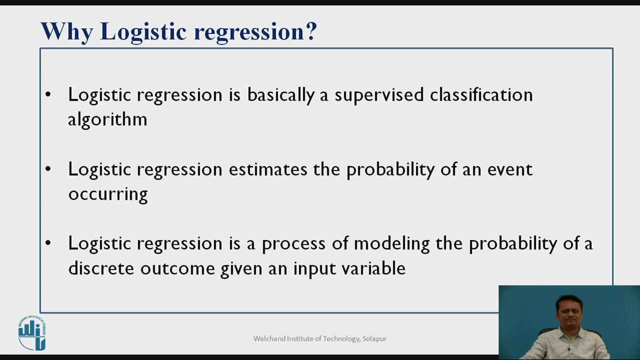 by a person and also student will be able to analyze the performance of the logistic regression for that insurance data. Basically, why we use the logistic regression: Logistic regression can be used for a supervised learning application called as classification. Basically, what logistic regression does: 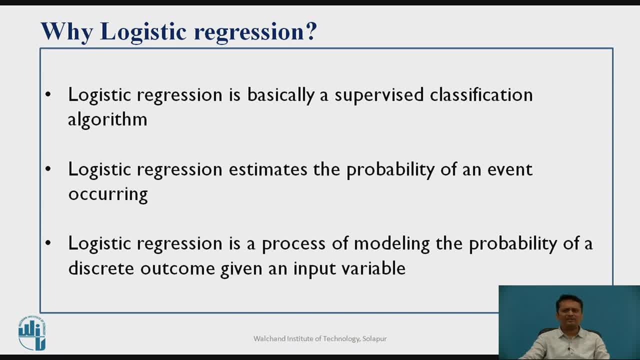 is. it tries to calculate the probability of an event and if there are two possible outputs, if it is a binary classification problem, easily, if the probability is greater than 0.5, you may say that the instance belongs to one class, and if it is less than 0.5, you can say, or you may. 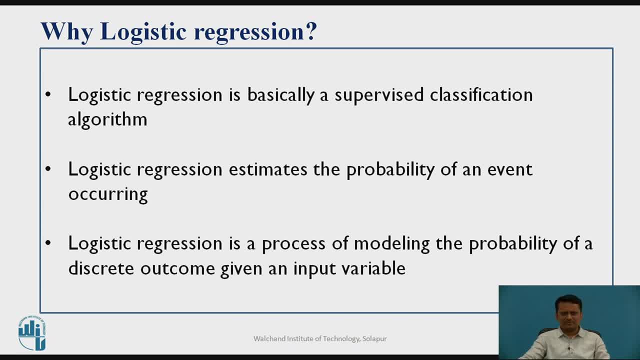 conclude that the instance belong to some other class. So basically, for binary classification, easily we can use this logistic regression approach. So summarizing, logistic regression is a process of developing a model based on the probability, and it models the probability of a discrete outcome given an input variable. 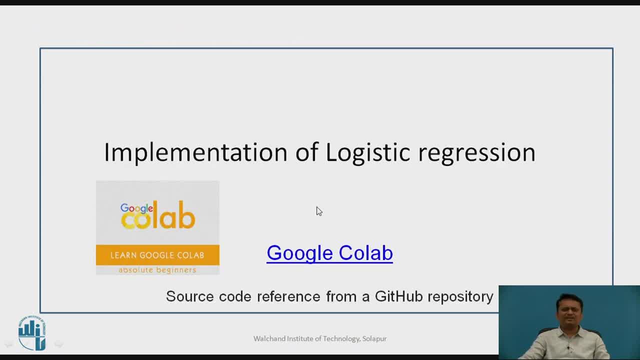 So let us try to understand the implementation of this logistic regression. A cloud-based google collaborative laboratory approach we will be using for the implementation, and the source codes are referred from the github repository as well. The data sets used for the code are taken from the Kaggle, so let us move to the implementation part. so when you 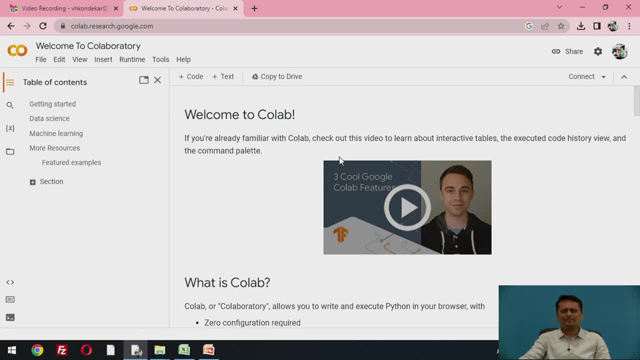 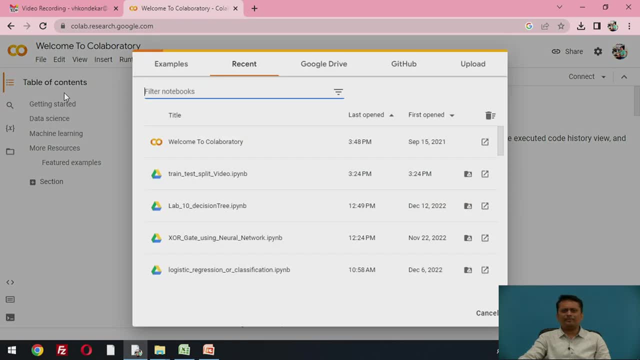 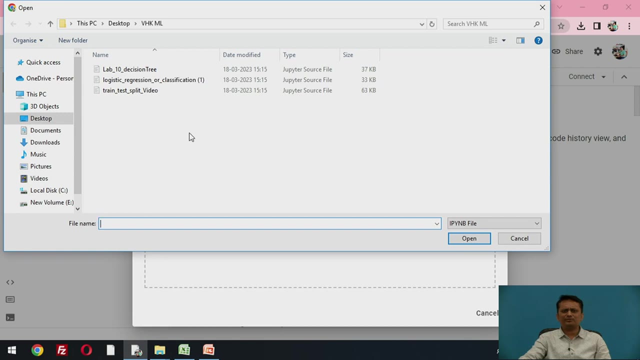 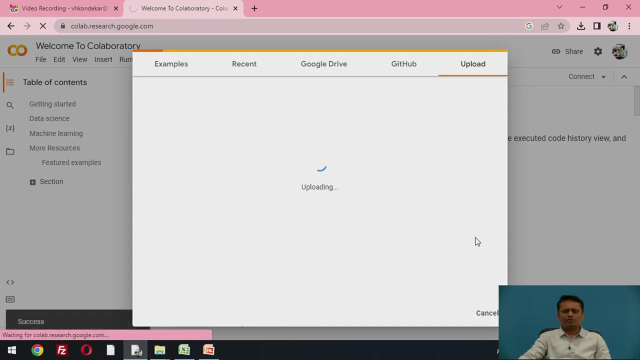 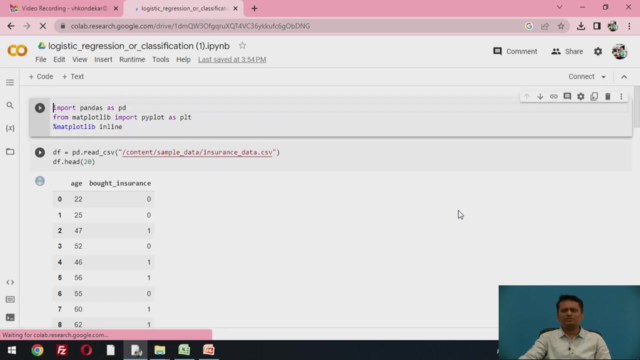 have that's Google collab platform open, you can execute your code. presently I have my Python notebook file available so I will be using that. so just give the path for that Python notebook file to the Python notebook file. whatever data set you are using for the program, that data set should be also made available. 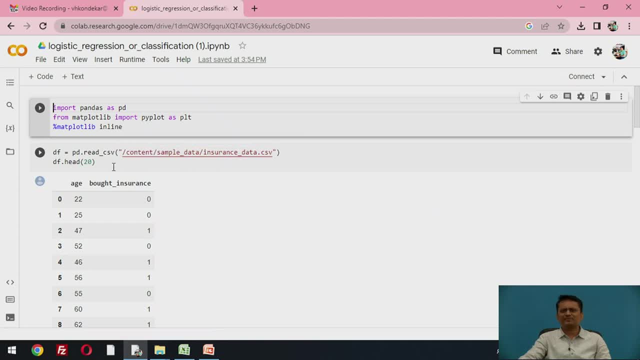 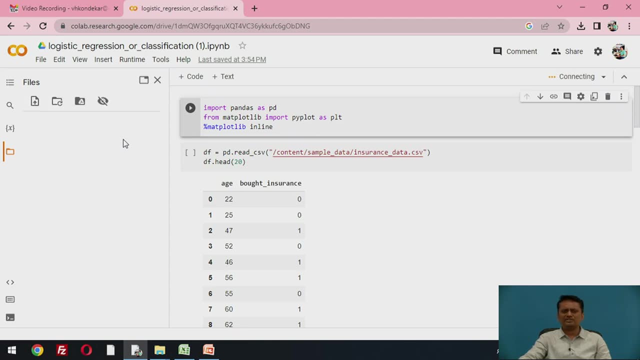 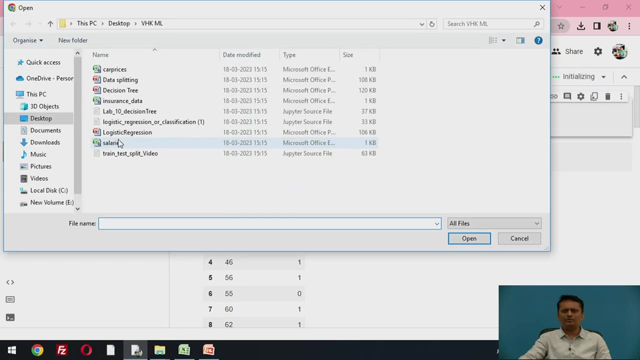 so we require insurance data set here. so make sure that you are mentioning that insurance data set. you are providing that insurance data set onto the cloud platform, so in the default folder called as sample data set. you are providing that insurance data set onto the cloud platform, so in the default folder called as sample data. I will upload, upload that. 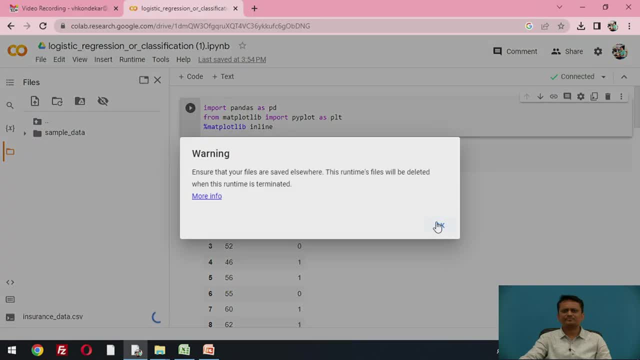 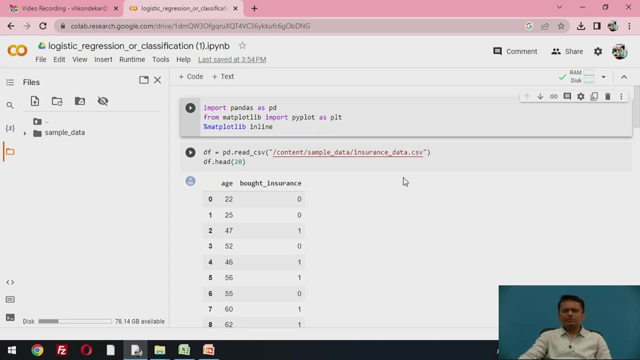 sample data. I will upload. upload that sample data. I will upload. upload that insurance data file- now the file is ready. insurance data file: now the file is ready. insurance data file: now the file is ready. so file is available in the CSV format. so file is available in the CSV format. 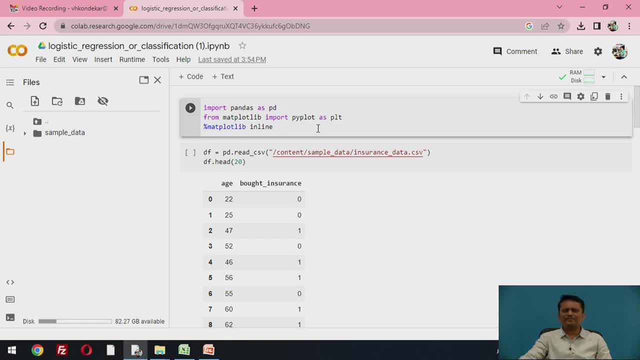 so file is available in the CSV format. and to read that file, so you will be. and to read that file, so you will be. and to read that file, so you will be. importing a library called as pandas, importing a library called as pandas, importing a library called as pandas, also to have some visualizations, we will. 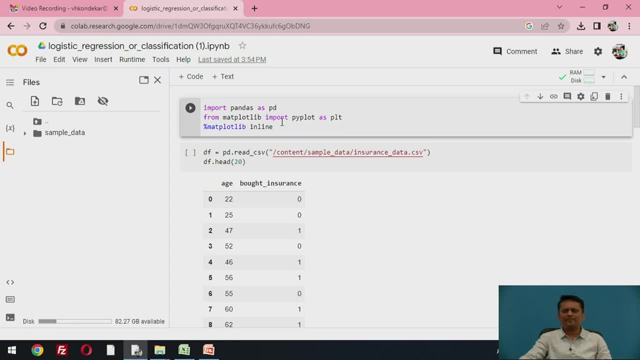 also to have some visualizations. we will also to have some visualizations. we will import a library, import a library, import a library called as matplotlib and the results of the library called as matplotlib and the results of the library called as matplotlib and the results of the library matplotlib. whatever visualizations are. 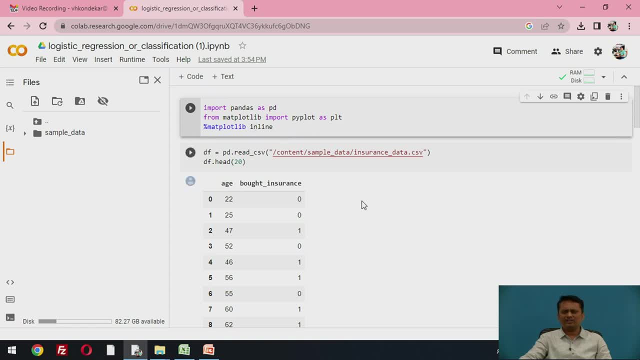 matplotlib. whatever visualizations are, matplotlib, whatever visualizations are there, so those visualizations you want in there, so those visualizations you want in there, so those visualizations you want in this particular collab file itself, so this particular collab file itself, so this particular collab file itself. so it's made in line. so whatever results. 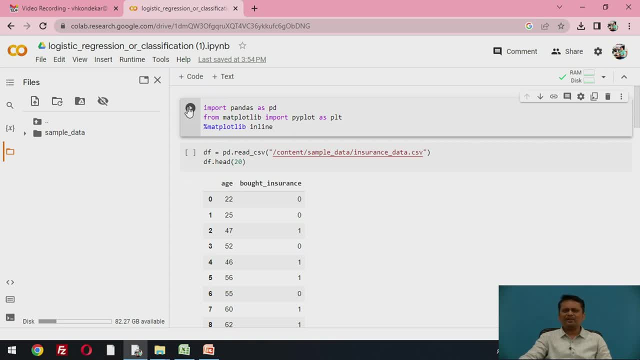 it's made in line, so whatever results it's made in line, so whatever results will be visualized here itself. so now let will be visualized here itself. so now let will be visualized here itself. so now let me run, start running the code. so the 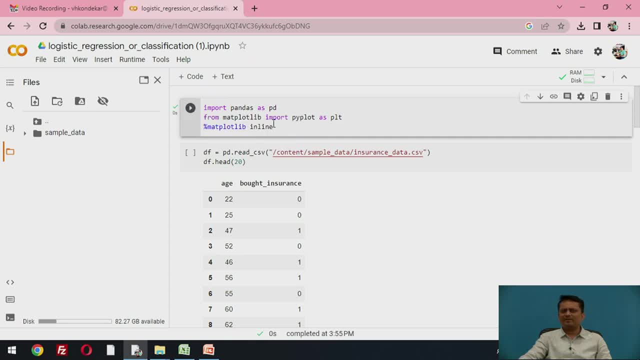 me run. start running the code. so the me run. start running the code. so the files will be imported now. library files will be imported now. library files will be imported now. library files: now you will be reading the CSV file. so files: now you will be reading the CSV file. so 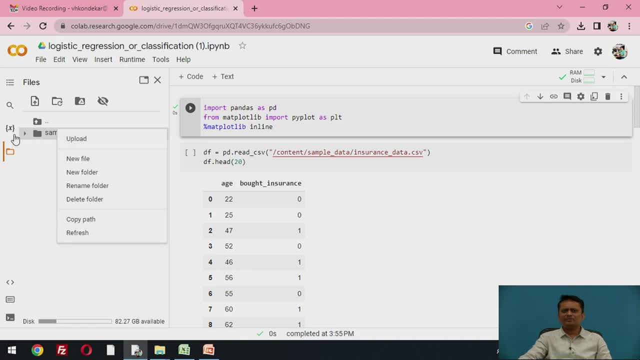 files. now you will be reading the CSV file. so when you are imported the file, so when you are imported the file, so when you are imported the file, so the file will be available here. so make, the file will be available here. so make, the file will be available here. so make sure that, whatever path you are having, 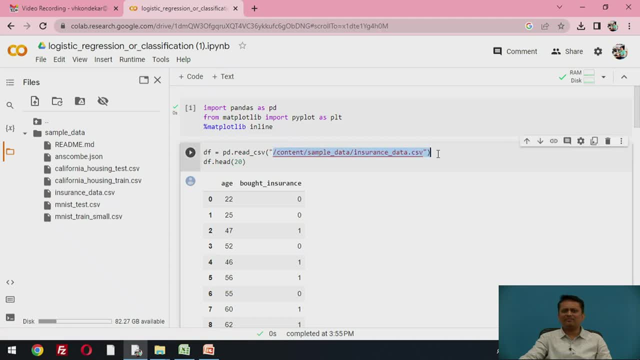 sure that whatever path you are having, sure that whatever path you are having, so the same path you are providing here, so the same path you are providing here, so the same path you are providing here. when you are reading that CSV, so you, when you are reading that CSV, so you. 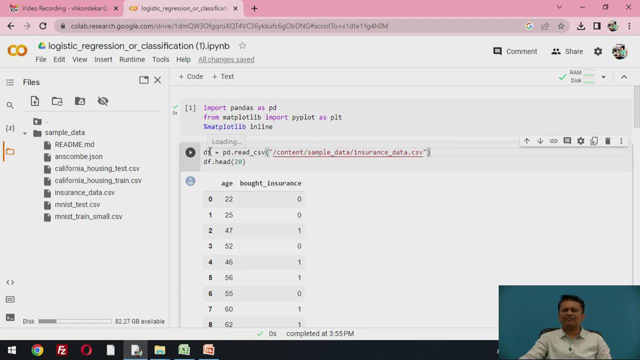 when you are reading that CSV. so you read that CSV and CS will be stored in a read. that CSV and CS will be stored in a read. that CSV and CS will be stored in a data frame called as a DF. now, if you data frame called as a DF. now, if you. 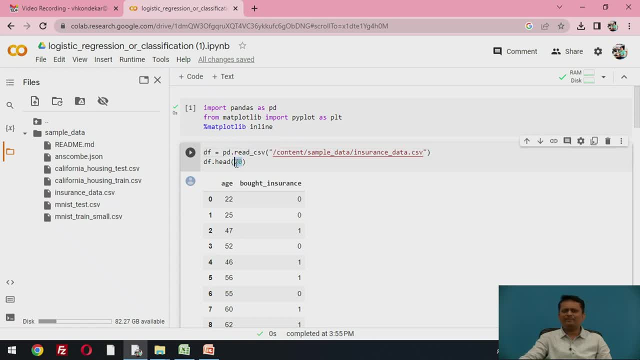 data frame, called as a DF. now, if you want to view what exactly you have in, want to view what exactly you have in, want to view what exactly you have in data frame, so by default if you just put data frame, so by default if you just put. 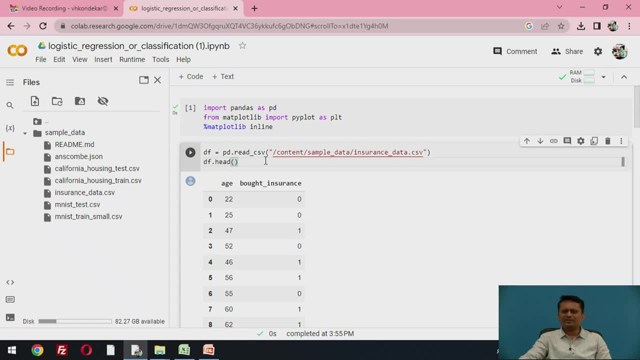 data frame. so by default, if you just put DF dot head, you're calling that function. DF dot head, you're calling that function, DF dot head, you're calling that function. so it will give you by default first. so it will give you by default first. so it will give you by default first five rows of the data and if you want to, 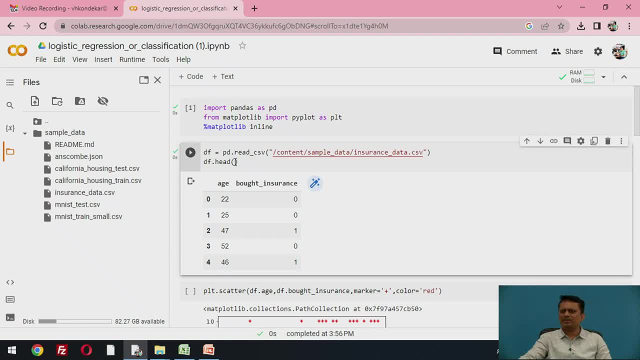 five rows of the data. and if you want to, five rows of the data, and if you want to have visualization of few more rows, so have visualization of few more rows. so have visualization of few more rows. so that number you can mention over here, so that number you can mention over here. so 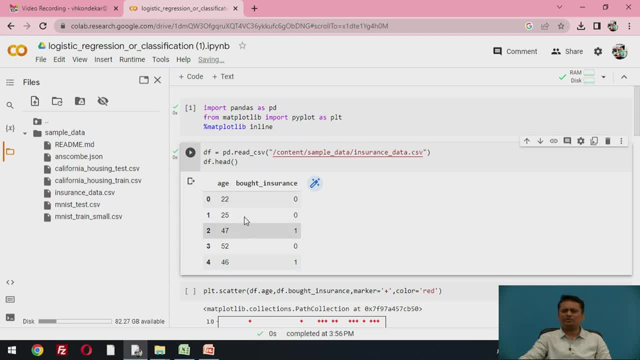 that number you can mention over here. so what simple data I am having is there. what simple data I am having is there? what simple data I am having is there are two attributes. one is called as the are two attributes. one is called as the are two attributes. one is called as the H, or the person, and then the target. 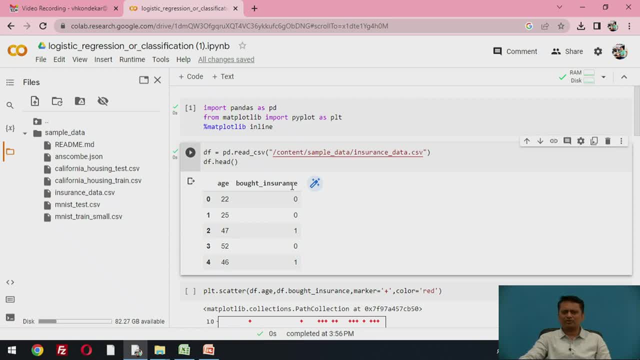 H or the person, and then the target: H or the person. and then the target attribute is whether that person has. attribute is whether that person has. attribute is whether that person has brought the insurance or not. zero brought the insurance or not. zero brought the insurance or not. zero indicates person hasn't brought the. 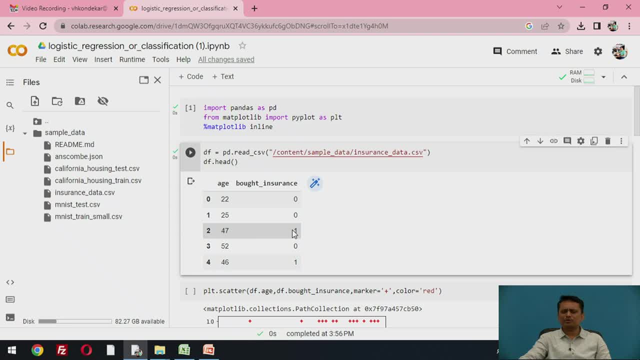 indicates person hasn't brought the indicates person hasn't brought the insurance and one indicates person is insurance and one indicates person is insurance and one indicates person is positive person has taken that insurance. positive person has taken that insurance. positive person has taken that insurance. so this is the insurance data we are. 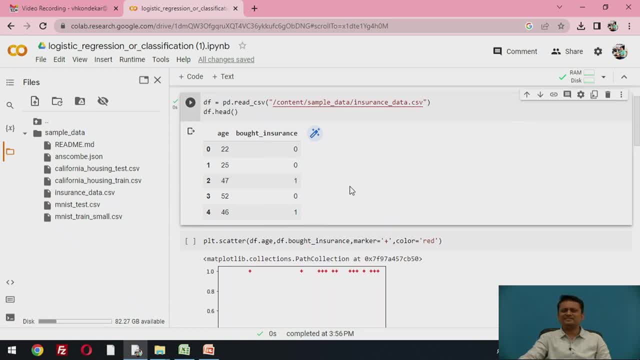 so this is the insurance data we are. so this is the insurance data we are having. let us try to visualize this data having. let us try to visualize this data having. let us try to visualize this data so by varied visualization can be done. so by varied visualization can be done. 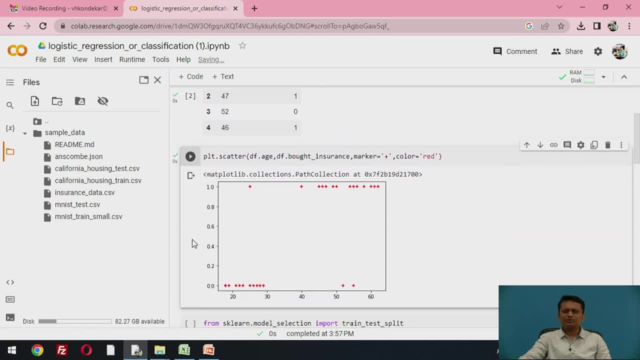 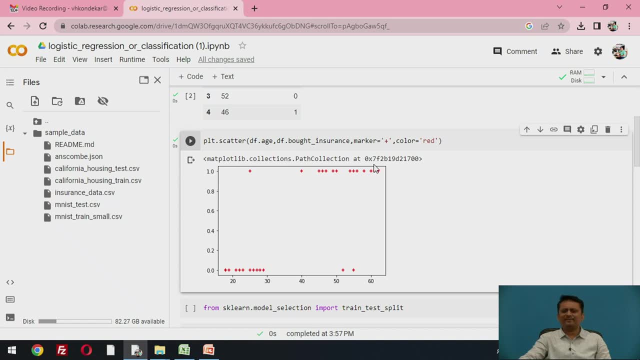 so by varied visualization can be done by having a scatter plot. so I am having by having a scatter plot. so I am having by having a scatter plot, so I am having this scatter plot and all the instances, this scatter plot, and all the instances, this scatter plot and all the instances in your data are visualized here. so if 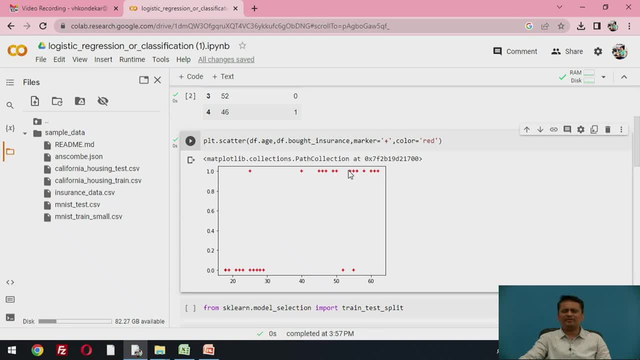 in your data are visualized here. so if in your data are visualized here, so if you look at this particular data split, you look at this particular data split, you look at this particular data split, you'll understand that I cannot go for. you'll understand that I cannot go for. 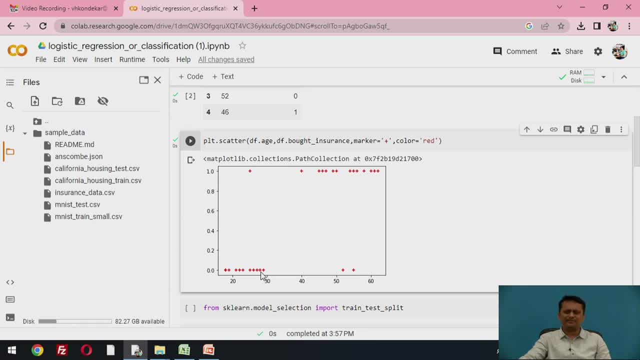 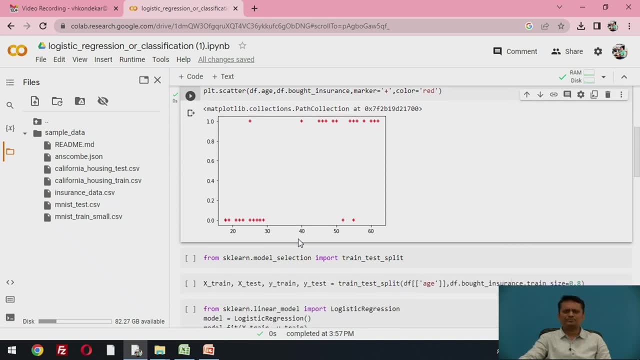 you'll understand that I cannot go for linear regression. I cannot represent linear regression. I cannot represent linear regression. I cannot represent this data by a single line and hence a this data by a single line and hence a this data by a single line and hence a logistic recreation approach can be used. 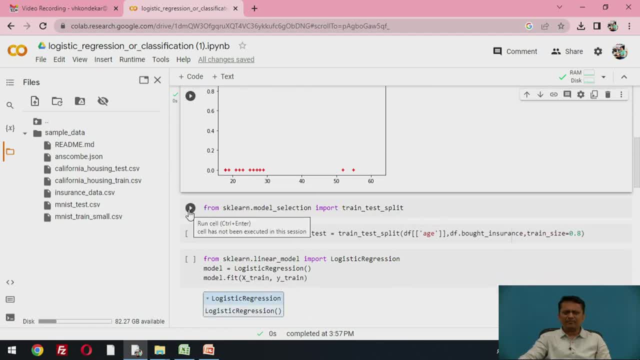 logistic recreation approach can be used. logistic recreation approach can be used. so again we are using the split of the. so again we are using the split of the. so again we are using the split of the data into the training set and testing. data into the training set and testing. 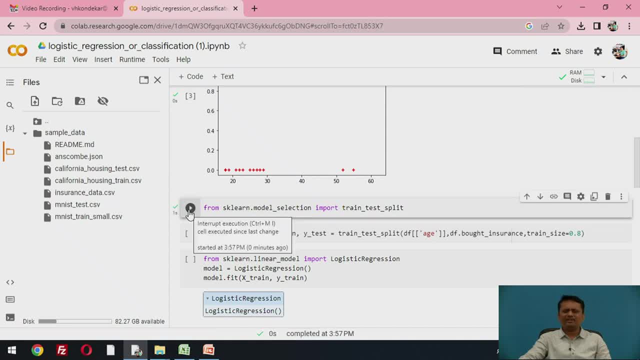 data into the training set and testing set. so for that we are using importing set. so for that we are using importing set. so for that we are using importing that library from scikit-learn and the that library from scikit-learn and the that library from scikit-learn. and the data split is done here with a training. 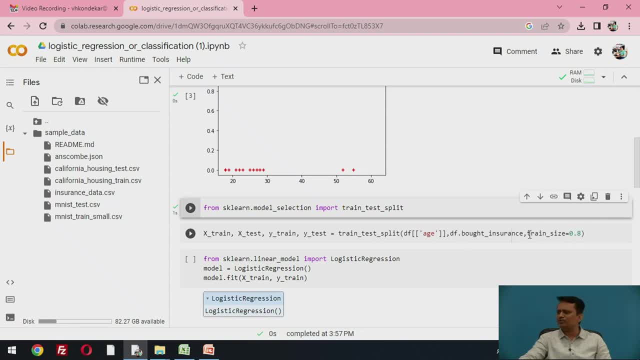 data split is done here with a training. data split is done here with a training size of 0.8. 80% data will be used for size of 0.8. 80% data will be used for size of 0.8. 80% data will be used for the training purpose and remaining 20%. 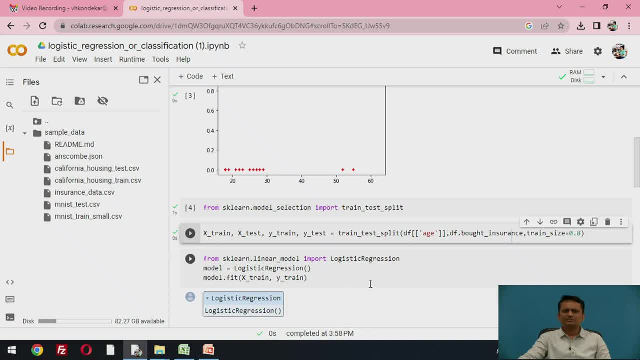 the training purpose and remaining 20%. the training purpose and remaining 20% data will be used for. the testing data will be used for the testing data will be used for the testing purpose. so split is done and the split purpose. so split is done and the split. 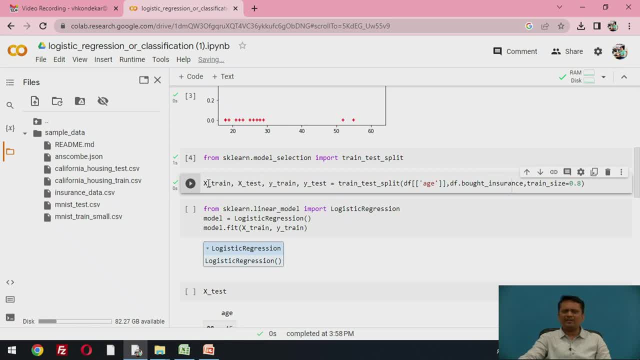 purpose. so split is done and the split will provide you four different values. will provide you four different values. will provide you four different values where inputs of the training data set, where inputs of the training data set. where inputs of the training data set will be available in extreme output of: 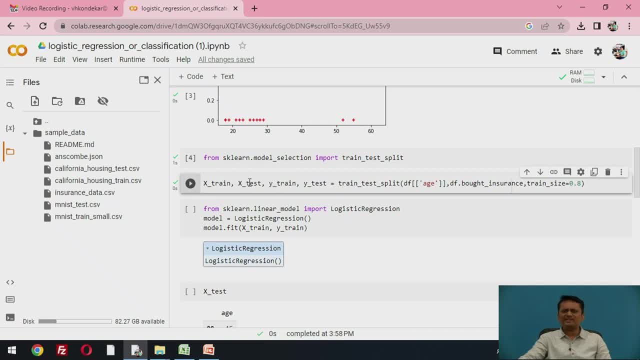 will be available in extreme output of. will be available in extreme output of: the training data set in y train input. the training data set in y train input. the training data set in y train input for the test data set in X test and for the test data set in X test. and. 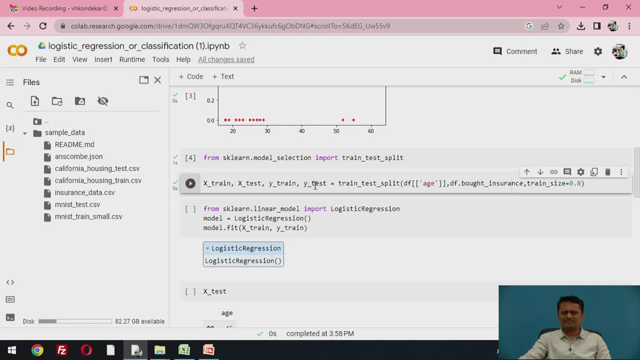 for the test. data set in X test and output of the text data set in y test. so output of the text data set in y test. so output of the text data set in y test. so this split is done, so now you can go for. this split is done, so now you can go for. 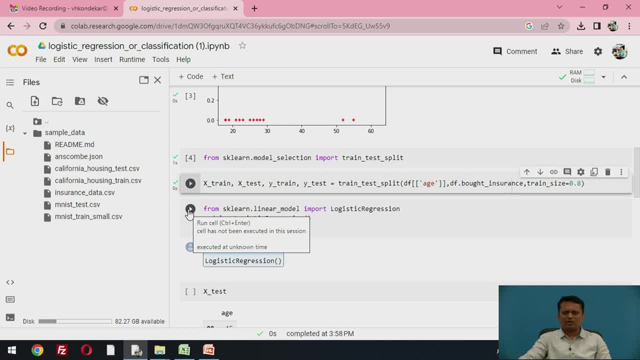 this split is done, so now you can go for developing a machine learning model. developing a machine learning model, developing a machine learning model, logistic regression model: you want to. logistic regression model. you want to. logistic regression model. you want to develop. and we all know that when you 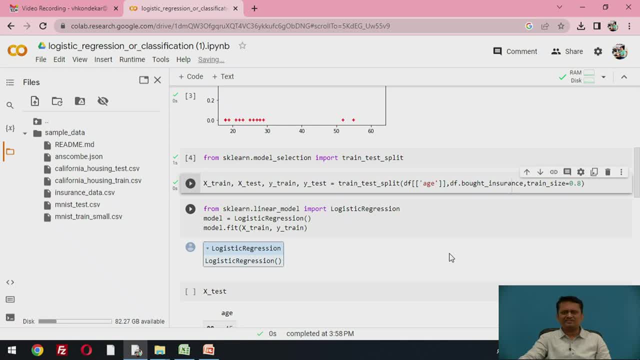 develop and we all know that when you develop, and we all know that when you are developing the model, if you are are developing the model, if you are are developing the model, if you are splitting the data into the training and splitting the data into the training and 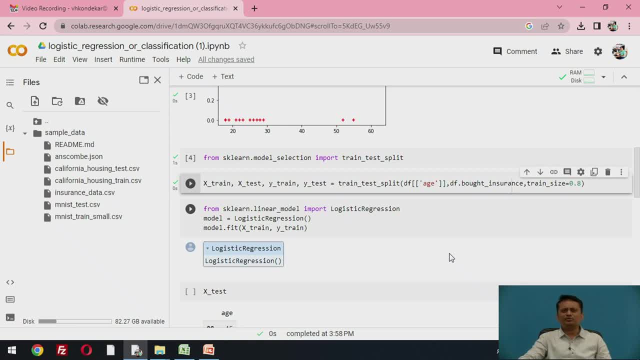 splitting the data into the training and testing data set. so training data set, testing data set. so training data set, testing data set. so training data set will be used for developing, the model will be used for developing, the model will be used for developing the model and test data set will be used to. and test data set will be used to and test data set will be used to: evaluate the performance of the model, evaluate the performance of the model, evaluate the performance of the model which has been developed by using the which has been developed by using the which has been developed by using the training data set. so here we are. 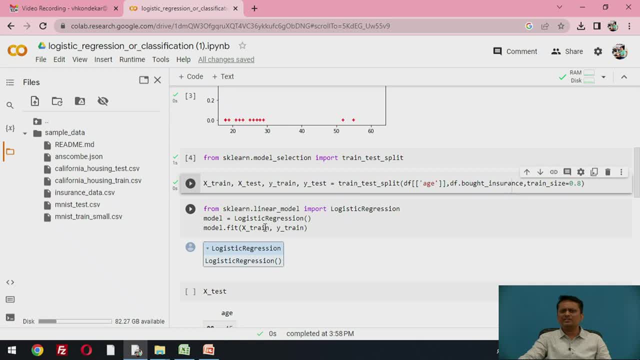 developing the model so law using this, developing the model so law using this, developing the model so law using this. extreme and white rain. so let us extreme and white rain. so let us extreme and white rain. so let us develop a model logistic regression model. develop a model logistic regression model. 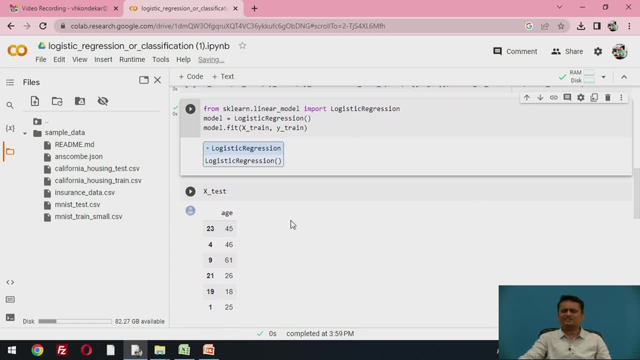 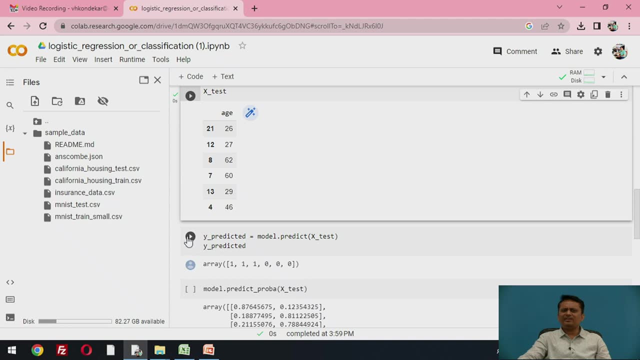 develop a model, logistic regression model. and now let us check what are the. and now let us check what are the. and now let us check what are the results. so actual test data set will be results. so actual test data set will be results. so actual test data set will be visualized here. then you will go on. 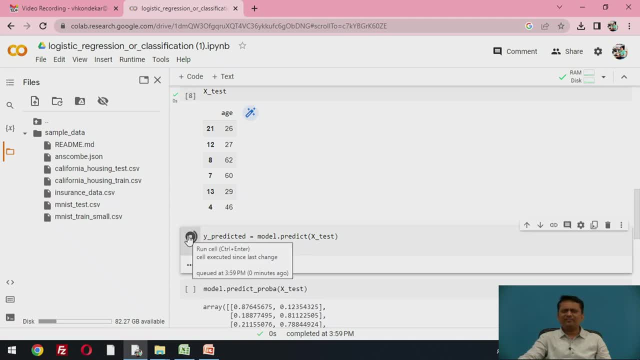 visualized here, then you will go on visualized here, then you will go on making the prediction that if these are making the prediction, that if these are making the prediction that if these are the values of the input of the age, the values of the input of the age, 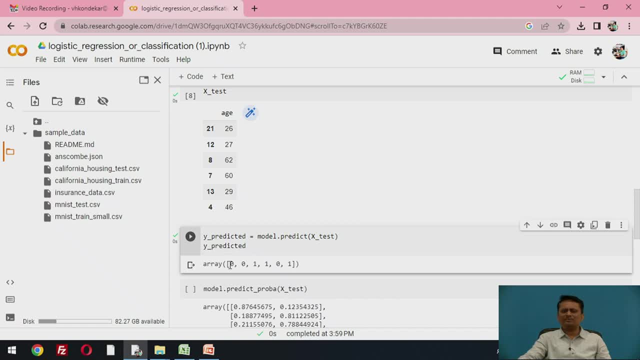 the values of the input, of the age, whether the person will go for the, whether the person will go for the, whether the person will go for the insurance or not. in terms of the insurance or not. in terms of the insurance or not. in terms of the probability values, it will be calculated. 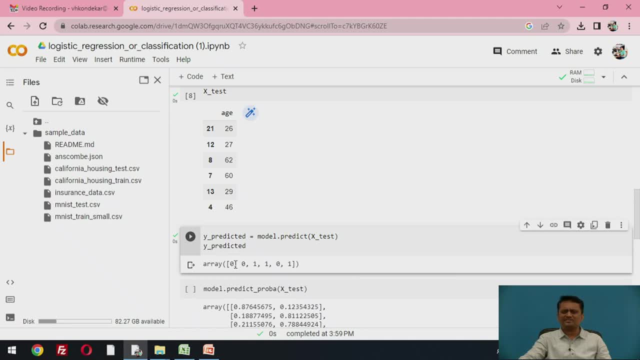 probability values: it will be calculated. probability values: it will be calculated, and then those probabilities are, and then those probabilities are, and then those probabilities are converted into the decision classes. so converted into the decision classes, so converted into the decision classes. so age 25. result is zero. miss person may: 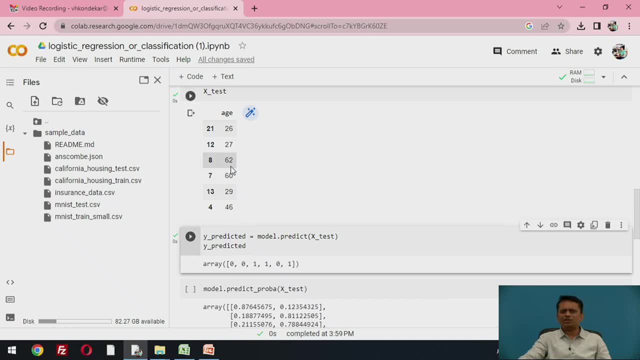 age 25. result is zero. miss person may age 25. result is zero. miss person may not go for the insurance but age 62 and not go for the insurance but age 62 and not go for the insurance but age 62 and 60, the persons will go for the insurance. 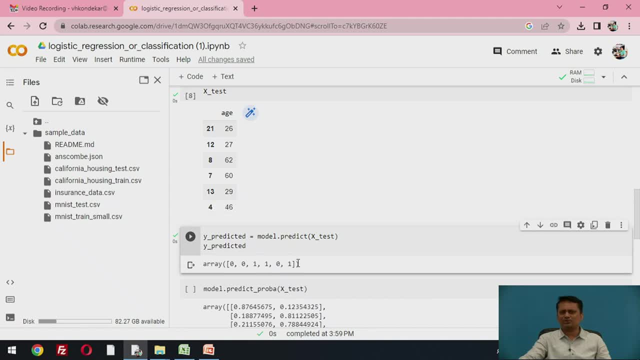 60: the persons will go for the insurance. 60: the persons will go for the insurance as well. age 46 person will go for the as well. age 46 person will go for the as well. age 46 person will go for the insurance. basically, whatever. 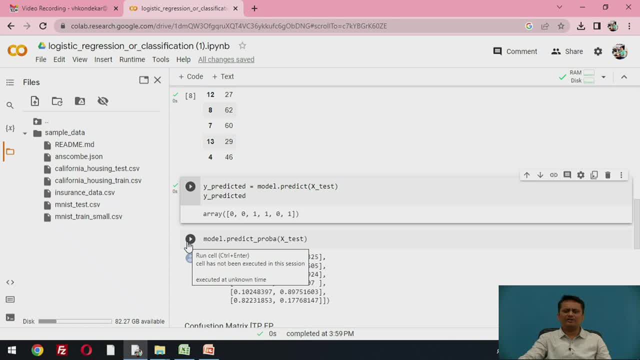 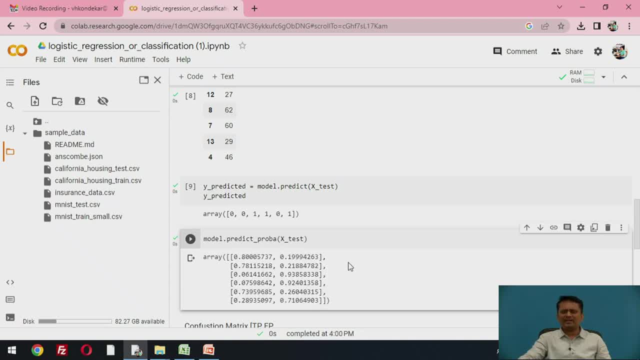 view so you can view these probabilities. view so you can view these probabilities. so, for the first input data set, that is so for the first input data set. that is so for the first input data set. that is the age value 25, what you are finding, the age value 25, what you are finding. 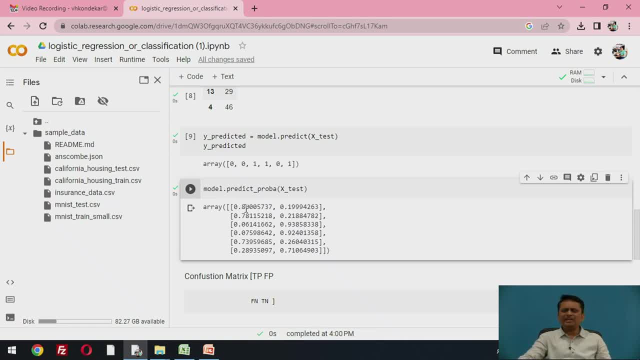 the age value 25. what you are finding here is around 80% probability is there. here is around 80% probability is there. here is around 80% probability is there. that person will not take insurance. this, that person will not take insurance. this, that person will not take insurance. this probability of not taking, and hence 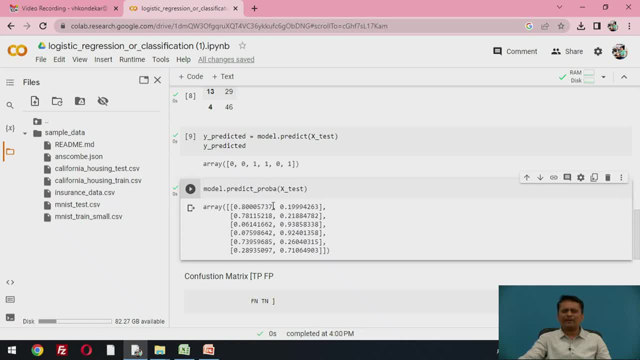 probability of not taking and hence probability of not taking, and hence this will be representing the probability of this, will be representing the probability of this will be representing the probability of taking the insurance. so if you taking the insurance, so if you taking the insurance, so if you compare these two values, you can come up. 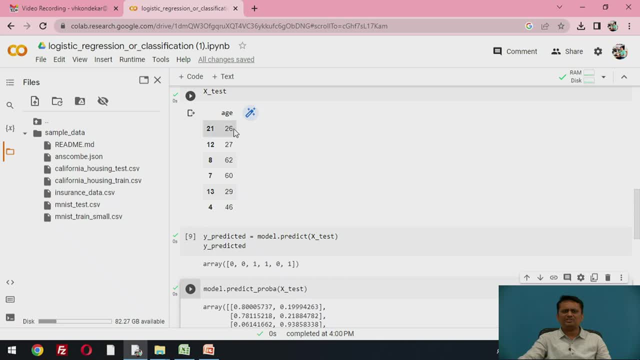 compare these two values, you can come up. compare these two values, you can come up with a conclusion that, if the age is 26, with a conclusion that if the age is 26, with a conclusion that if the age is 26, the logistic regression model developed. 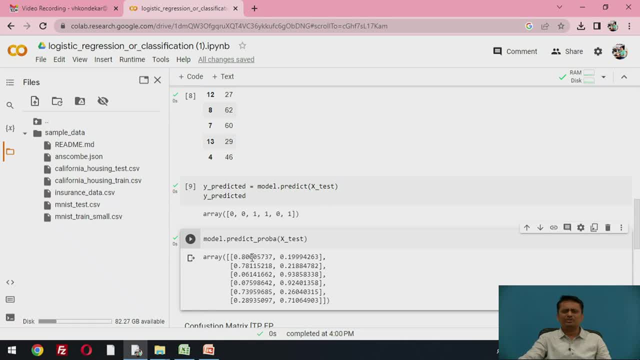 the logistic regression model developed. the logistic regression model developed: is more in favor of person will not take. is more in favor of person will not take. is more in favor of person will not take insurance. so that's why this prediction: insurance. so that's why this prediction. 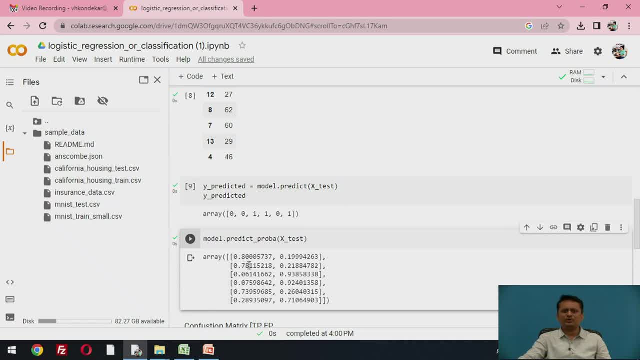 insurance. so that's why this prediction is 0 on the same lines here also. this is 0 on the same lines. here also, this is 0 on the same lines, here also. this problem, probability of not taking the problem, probability of not taking the problem, probability of not taking the insurance- is more. so prediction is 0 if. 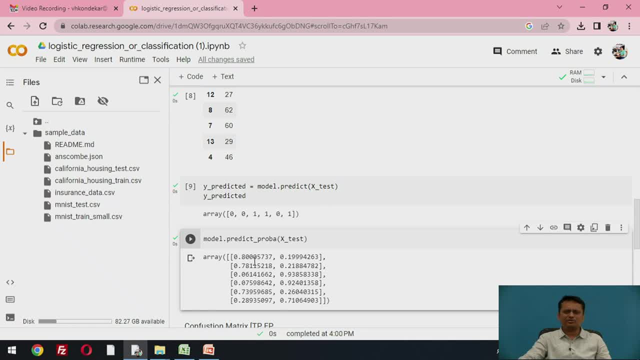 insurance is more so, prediction is 0. if insurance is more so, prediction is 0. if you look at here, it's 61%. so you'll say: you look at here, it's 61%. so you'll say: you look at here, it's 61%. so you'll say: it's a class 1 means person will take the. 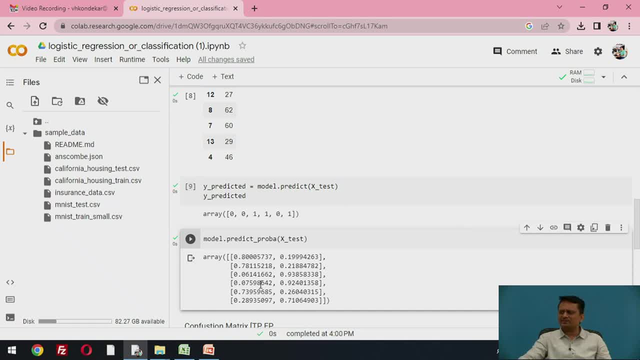 it's a class 1 means person will take the. it's a class 1 means person will take the insurance. same is true for next test insurance. same is true for next test insurance. same is true for next test data case. so around 92 percent data case, so around 92 percent. 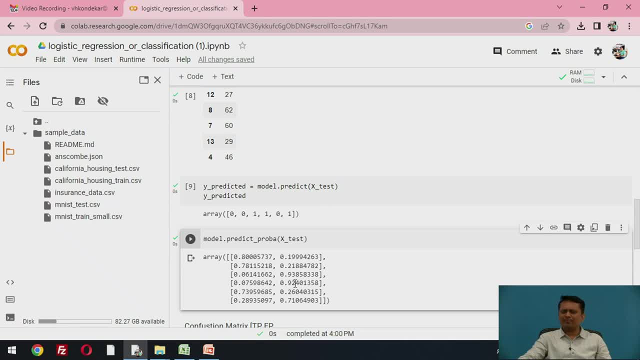 data case. so around 92 percent probability. you are getting of person probability. you are getting of person probability. you are getting of person taking insurance. so that's why the taking insurance. so that's why the taking insurance, so that's why the prediction is 1. so this is how you can. 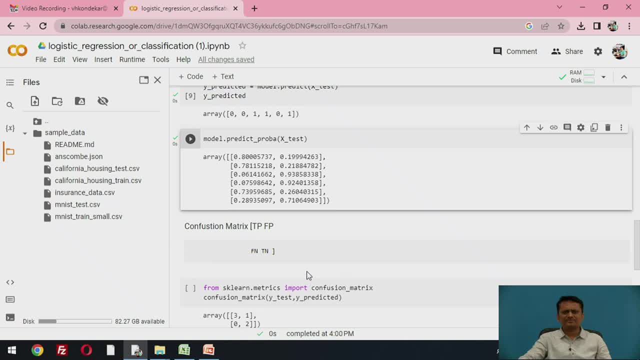 prediction is 1, so this is how you can. prediction is 1, so this is how you can. you can predict the results and you can. you can predict the results and you can. you can predict the results and you can classify the data into, in this case of 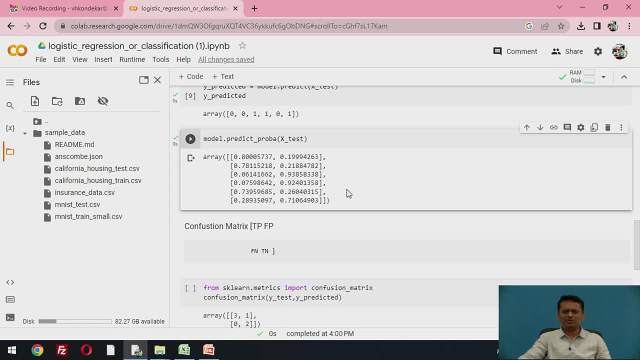 classify the data into, in this case of. classify the data into, in this case of problem: whether the person will take problem. whether the person will take problem, whether the person will take insurance or not. also the performance insurance or not. also the performance insurance or not. also the performance can be evaluated by having visualization of. 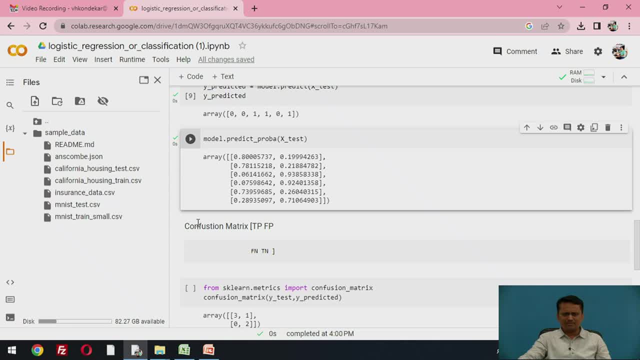 can be evaluated by having visualization of, can be evaluated by having visualization of the, or calculations of the confusion, the, or calculations of the confusion, the, or calculations of the confusion- matrix, and then later you may go for matrix, and then later you may go for matrix, and then later you may go for calculating different parameters. 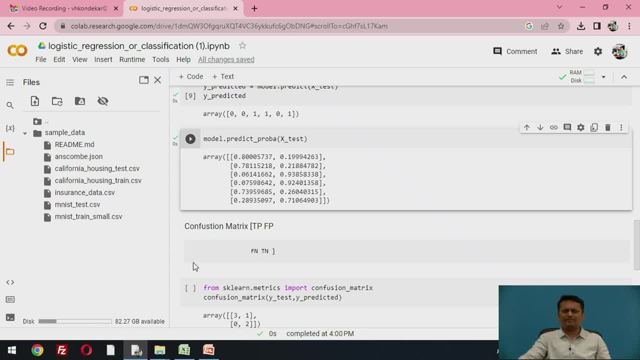 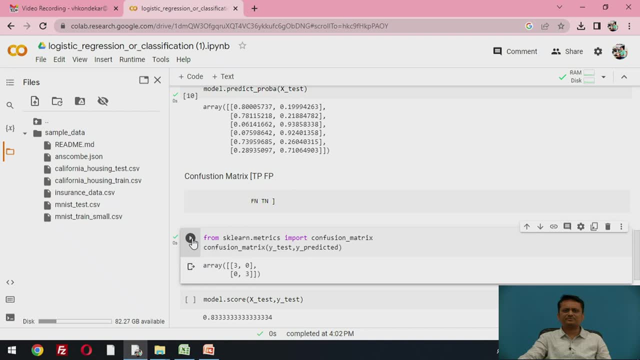 calculating different parameters, calculating different parameters of performance, from the confusion matrix of performance, from the confusion matrix of performance, from the confusion matrix itself. so you can have the itself, so you can have the itself, so you can have the visualization of the confusion matrix by, visualization of the confusion matrix by. 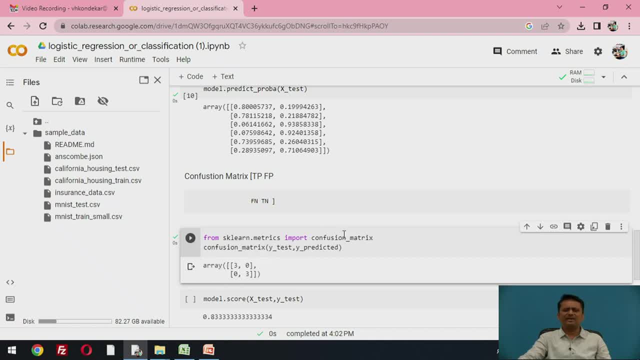 visualization of the confusion matrix by again importing this library of confusion, again importing this library of confusion, again importing this library of confusion matrix, and then this is what confusion matrix, and then this is what confusion matrix, and then this is what confusion matrix you are getting here, which is 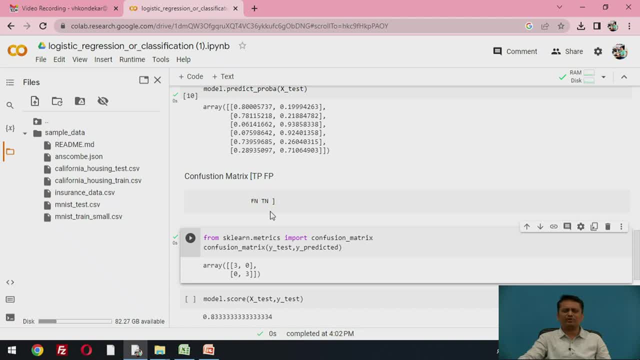 matrix. you are getting here which is matrix. you are getting here which is representing. so this is the representing, so this is the representing, so this is the representation of the confusion matrix, for representation of the confusion matrix, for representation of the confusion matrix for the two attributes. so these diagonal 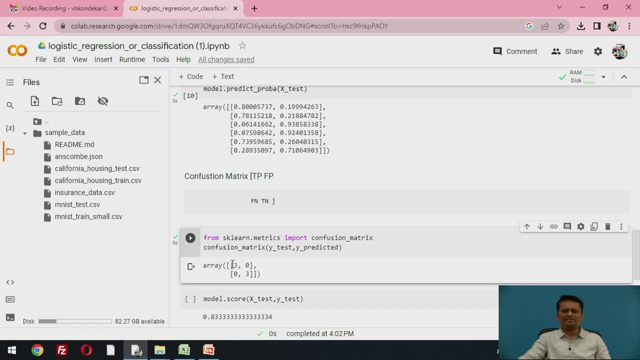 the two attributes. so these diagonal, the two attributes, so these diagonal elements are representing true positive elements, are representing true positive elements, are representing true positive and true negative and all the instances and true negative and all the instances and true negative and all the instances are represented in the diagonal part. 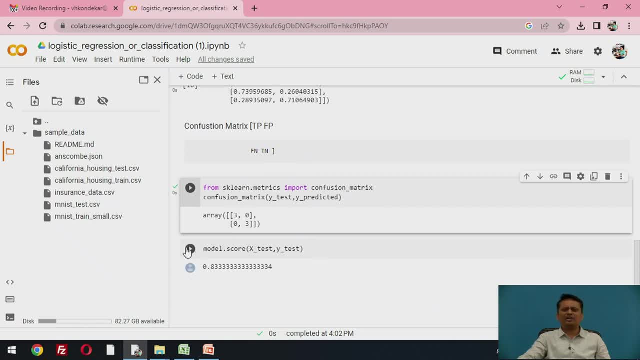 are represented in the diagonal part, are represented in the diagonal part itself means now the model model score itself. means now the model model score itself. means now the model model score will be hundred percent. model score will will be hundred percent. model score will will be hundred percent. model score will be hundred percent. now you can have a. 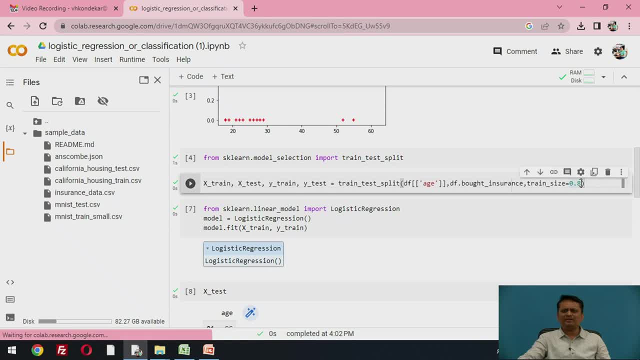 be hundred percent now you can have a be hundred percent now. you can have a different, different split, and then you different, different split, and then you different, different split, and then you may get the different confusion matrix, may get the different confusion matrix, may get the different confusion matrix, as well as different score also. so if I 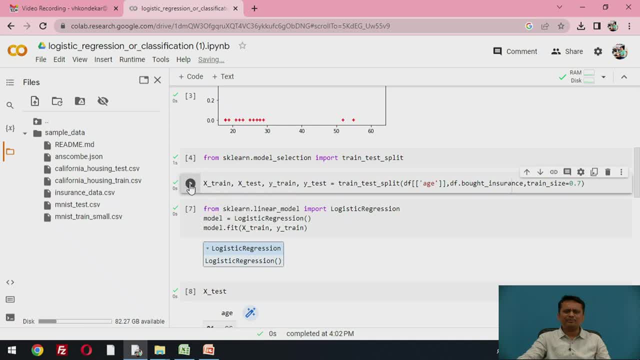 as well as different score also. so if I, as well as different score also. so if I make this point, seven means seventy. make this point: seven means seventy. make this point: seven means seventy. percent data set. I am using for the percent data set, I am using for the. 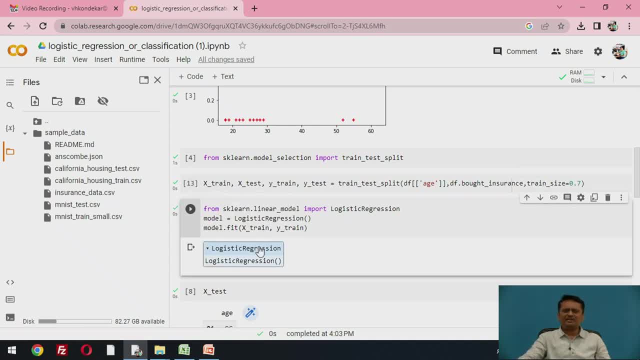 percent data set I am using for the training, and then that 70% data set I am training, and then that 70% data set I am training, and then that 70% data set I am using for developing the model. so again, using for developing the model, so again. 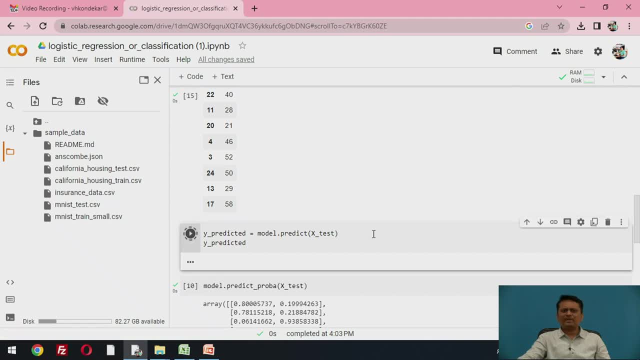 using for developing the model. so, again, the text data set will change based on the text data set will change based on the text data set will change. based on that, the predictions you need to make, that the predictions you need to make, that the predictions you need to make will be more, because test data set is. 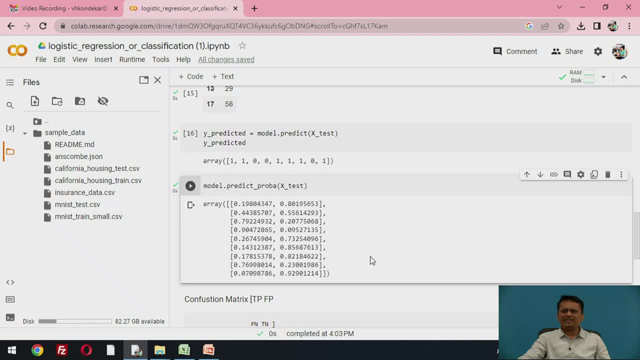 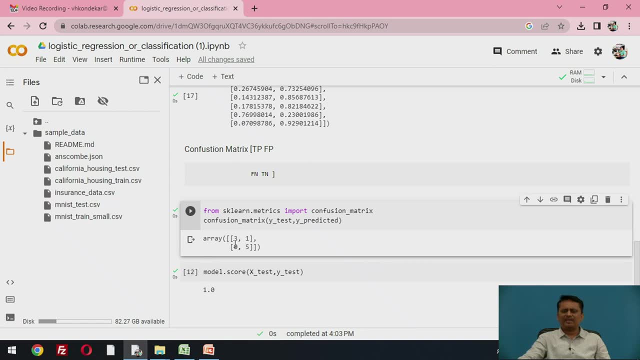 will be more because test data set is will be more because test data set is increase prediction in terms of the increase prediction, in terms of the increase prediction in terms of the probabilities. then again you can view the probabilities. then again you can view the probabilities. then again you can view the confusion matrix and, yes, some. 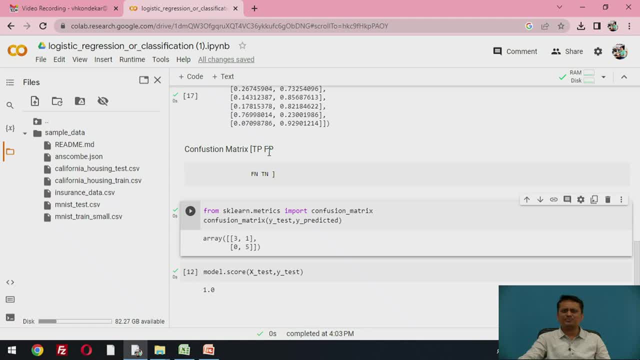 confusion matrix and, yes, some confusion matrix and, yes, some element are here. so there are some elements. element are here. so there are some elements, element are here. so there are some elements which are representing the false, which are representing the false, which are representing the false positive. so definitely score will not be. 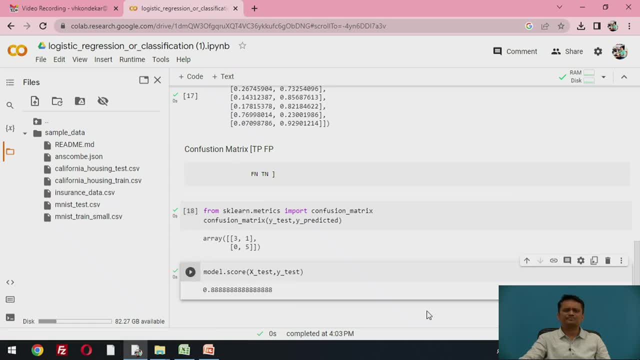 positive. so definitely score will not be positive. so definitely score will not be 100% here it will be reduced. so this is 100% here it will be reduced. so this is 100% here, it will be reduced. so this is how you can have a implementation of. 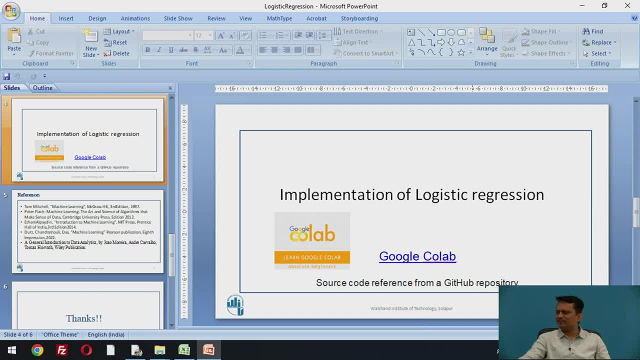 how you can have a implementation of, how you can have a implementation of logistic regression for the application, logistic regression for the application, logistic regression for the application called as classification, a supervised called as classification, a supervised called as classification, a supervised learning application, learning application, learning application. so. 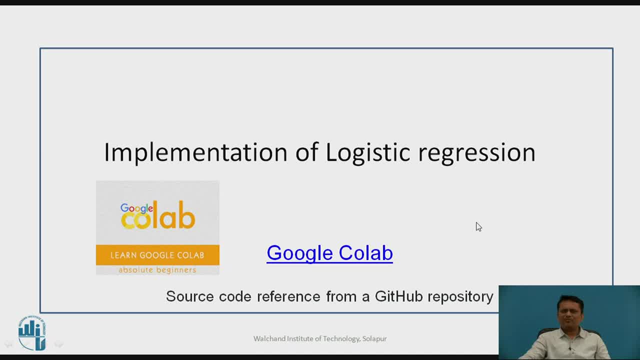 so this was the implementation of logistic. this was the implementation of logistic. this was the implementation of logistic regression through the Google Colab. you regression through the Google Colab, you regression. through the Google Colab. you can check the performance of the, can check the performance of the. 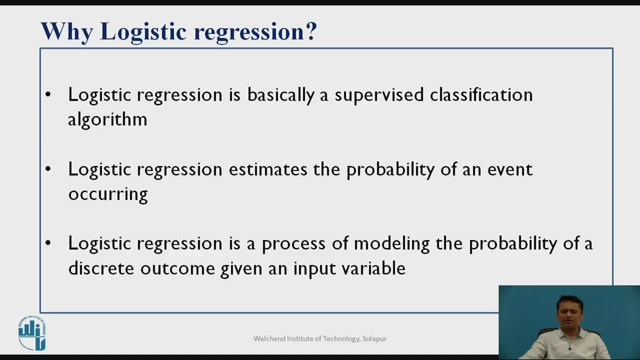 can check the performance of the algorithm for different values of algorithm. for different values of algorithm. for different values of different percentage of split. for the different percentage of split, for the different percentage of split for the train and test part. these are the train and test part. these are the. 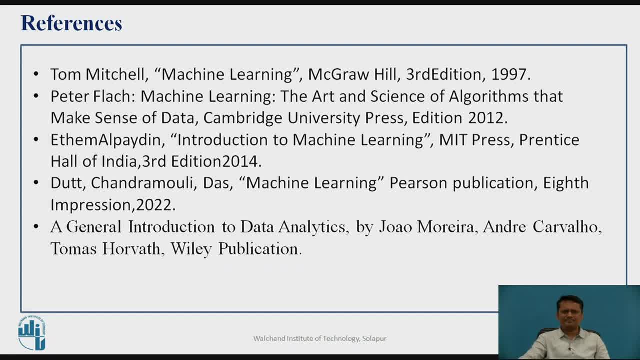 train and test part. these are the various references used for this video. various references used for this video. various references used for this video: presentation, presentation, presentation, presentation. thank you, thank you.